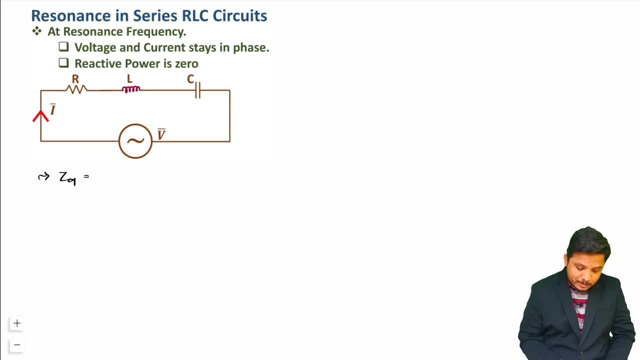 So here equivalent impedance, that will be series combination of impedance of R, L and C. So R is having impedance R, then L is having impedance XL, then capacitance C is having impedance XC. Now, my dear students, here R is real component only, but with inductor impedance will be J, omega. 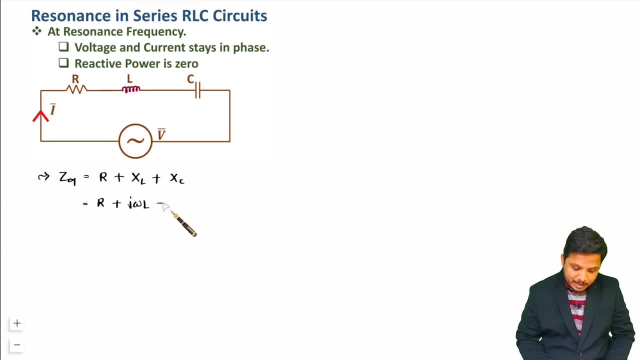 L, and with capacitor impedance will be plus 1 by J, omega C. Now here let us take real and imaginary part separately. So here V have real part, that is r, and if you take plus j over here- common from both of these terms- then 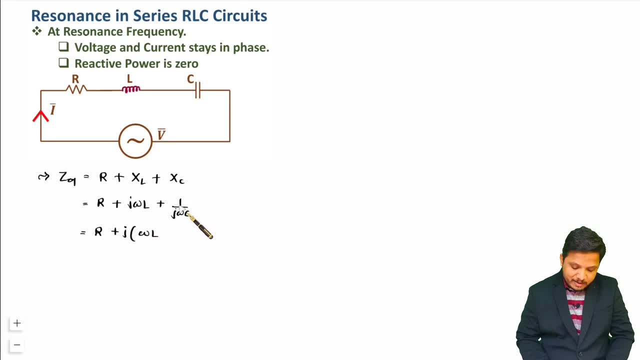 here we will be having omega l and in numerator j will be minus, so here minus 1 by omega c. so that is what impedance which we have with this series rlc circuit. now, my dear students, if you observe here this real component, so that is frequency independent, and if you observe this imaginary, 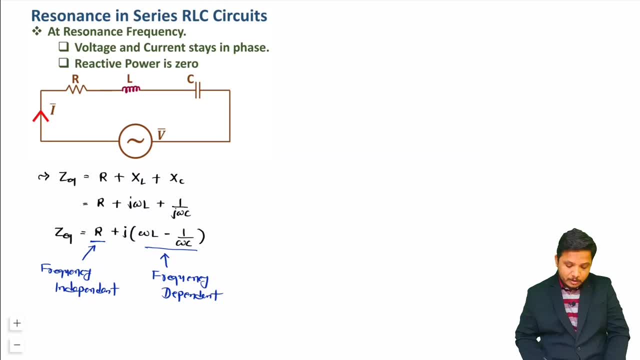 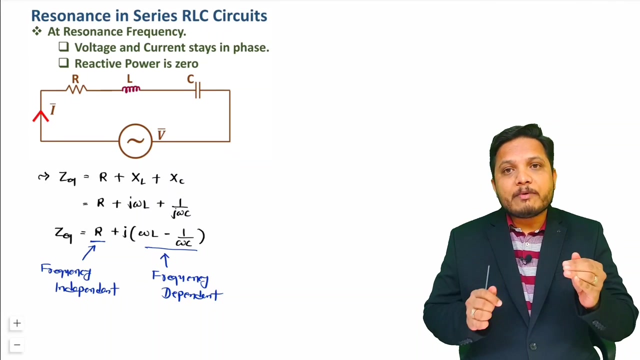 component that is frequency dependent. so here, this real component will not change, even if you change frequency of this ac supply, but as if you change frequency, then here you will be observing this imaginary component that will vary. so, my dear students, what is that which we are dealing to observe here? here we will be changing frequency and by changing frequency, 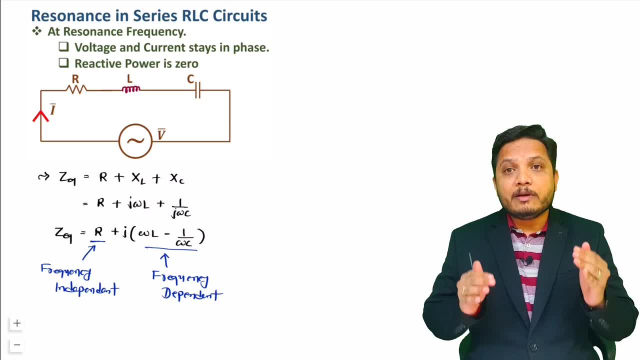 we will analyze how voltage and current phase are happening with each other, and as if voltage and current both are having same phase. then you can say there is a resonance now here, real component, that is frequency independent, and imaginary component, that is frequency dependent. so as frequency dependency is, 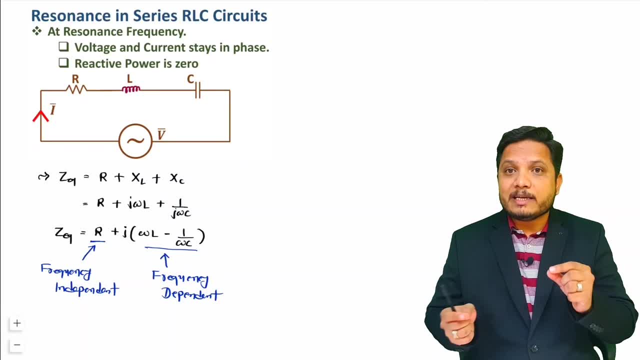 there with imaginary component. all you can do is by changing frequency. you can make imaginary component of impedance that will be zero, and as if you provide that, in that case what will happen? there will be only real component that is r. so in that case you can say voltage and current, that 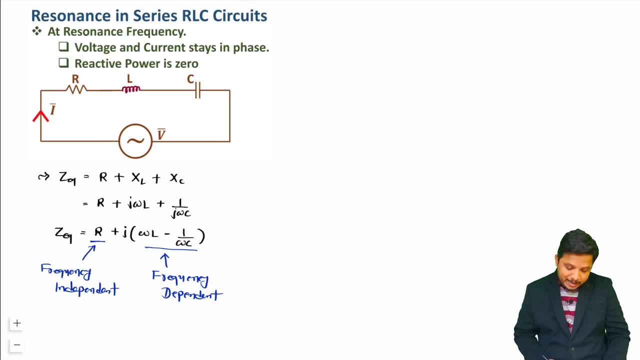 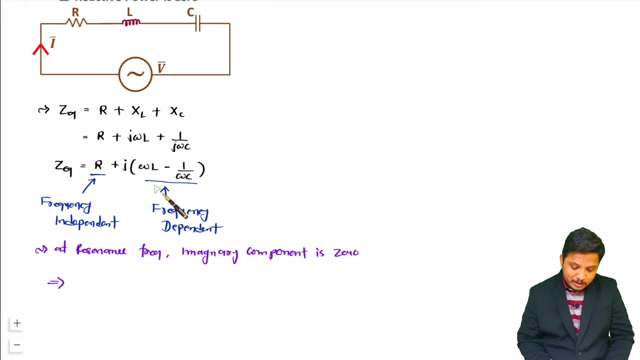 will get in same phase. so here, my dear students, if you observe this frequency dependent component that we are delivered to make zero by changing frequency, omega so as imaginary component is zero at resonant frequency, you will be having omega l minus one by omega c. that will be zero and 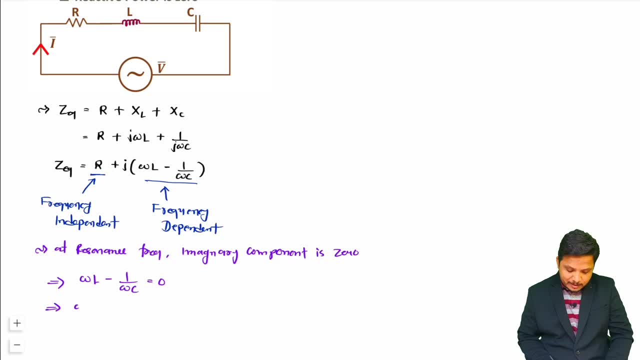 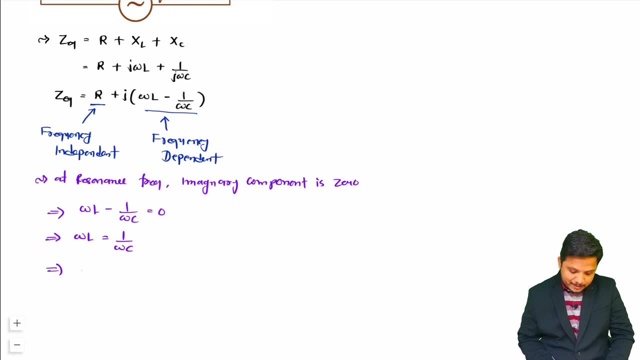 here you can simplify this so you can have: omega l is equals to one by omega c. so based on that you can say: omega square, that is 1 by LC. So I can say resonant frequency omega, that will be 1 by square root of LC. and 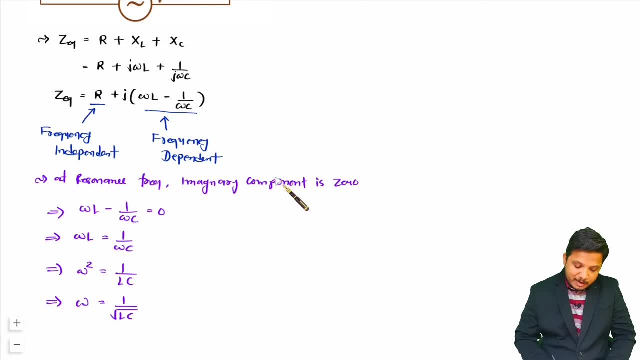 here you see, it is making this imaginary component 0.. So if you change omega in such a way that its value is 1 by square root of LC, in that case imaginary component will be 0, and as if imaginary component is 0, your impedance will be only resistive impedance. and for resistive impedance. 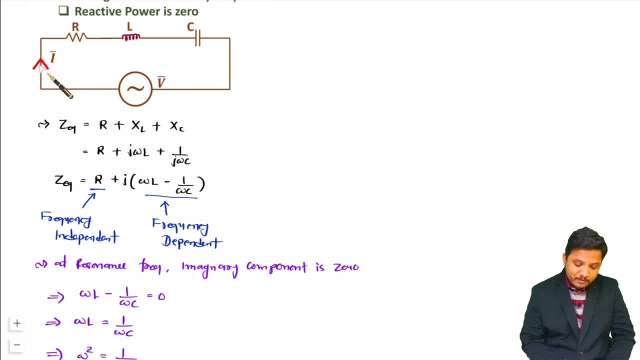 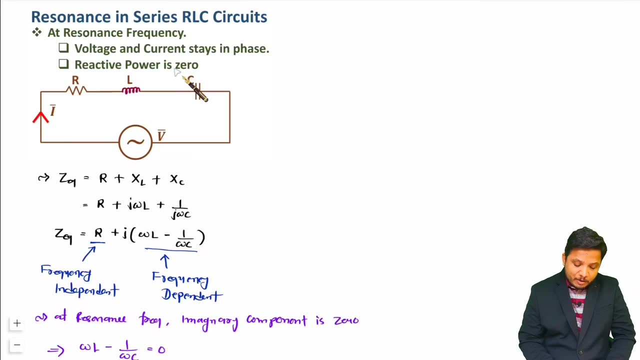 you should know voltage and current that will remain in same phase and as if it is remaining in same phase, reactive power will be 0 and as if reactive power is 0, only power will get dissipated across this resistor R and in that situation you will be having only real power in the network. 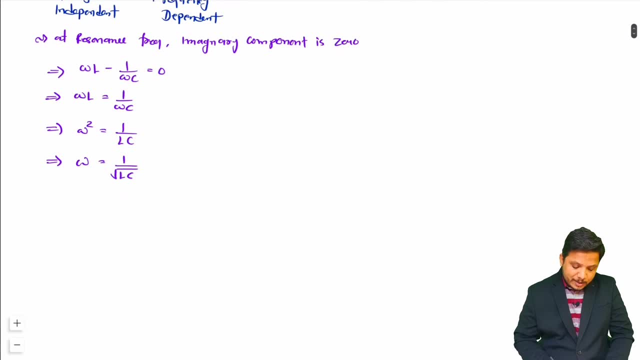 Now, my dear students, here, there are few essential key things that you should know, like this, Like this: resonant frequency unit is radian per second. Sometimes it may be given to you. in terms of frequency, then that will be 1 by 2 pi square root of LC, and that is there in terms of hertz. 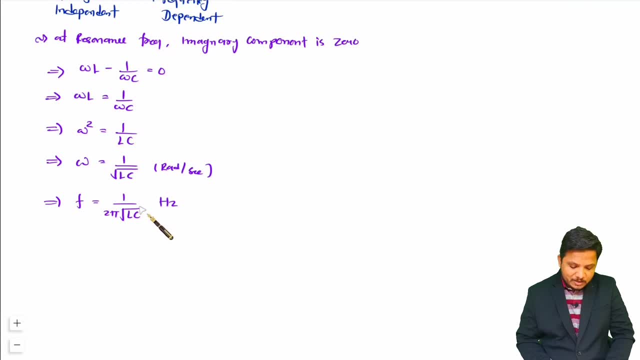 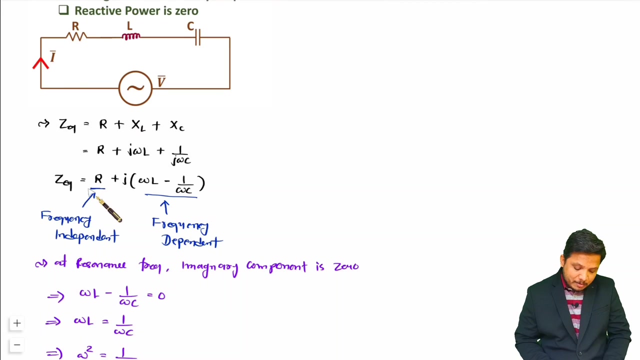 So you should see what is the unit which is given to you. based on that, you should calculate resonance. Now, my dear students here, when resonance is happening at that time, let us try to understand how much current is happening. So you see, as impedance is getting minimum technically, if you observe. 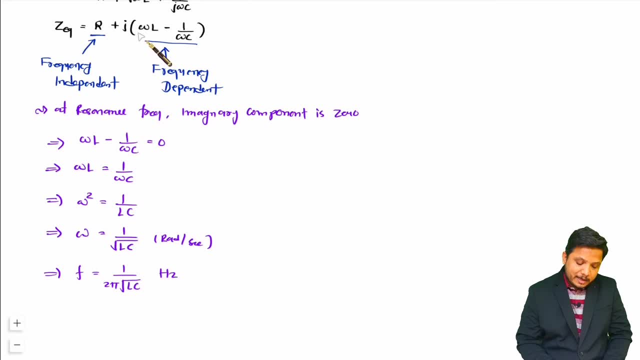 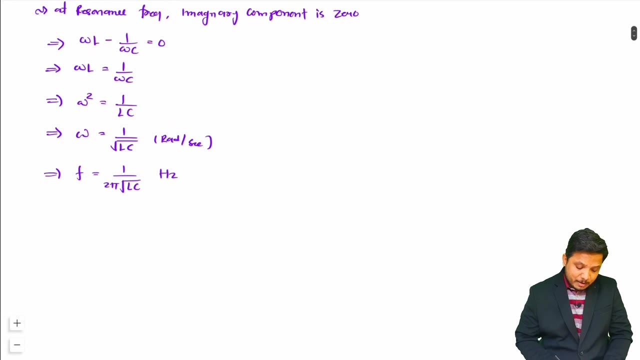 this Z equivalent, that is R plus J, into omega L minus 1 by omega C. but at resonance this component is 0, so impedance will be minimum impedance. So as if impedance is minimum, what will happen? Current will get maximum, So as Z equivalent, that is. 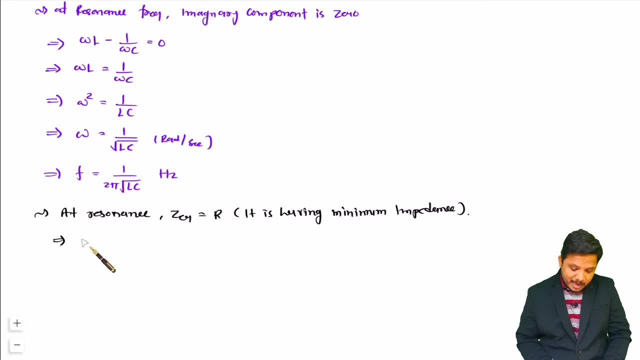 R only. our impedance will be minimum. So you will be having Z equivalent. that is R as well. as if you want to find what is the value of current, then that is V by Z. here Z is R. So I can say value of current, that will be maximum and that will be V by R. So at resonance maximum current will be V by. 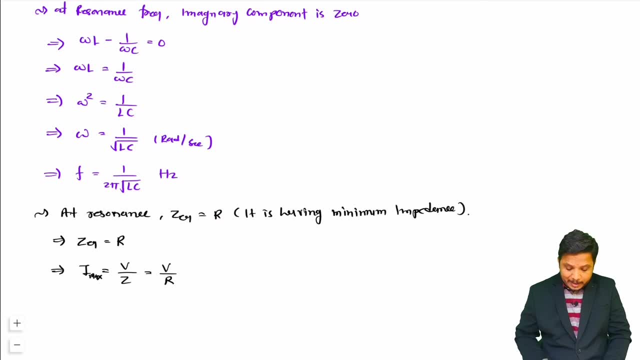 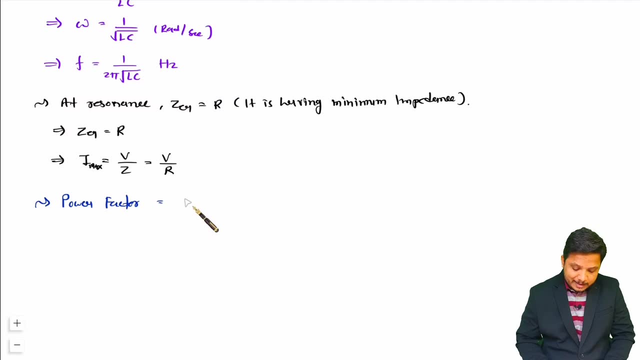 R, that you should know, and you should know what will be power. So you should know what will be power, Power factor here, my dear students. So power factor that is cos phi, and power factor that is R by Z, and here impedance is R only. 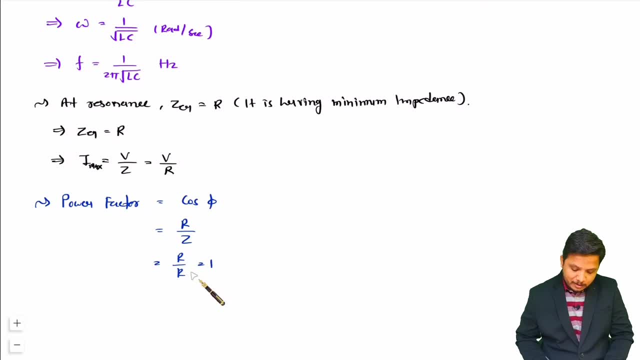 So I can say: R by R, that is equals to 1.. What it means Phase is 0.. What it means Phase in between voltage and current, that is 0.. So as phase in between voltage and current, that is 0.. So, as phase in between voltage and current, that is 0. 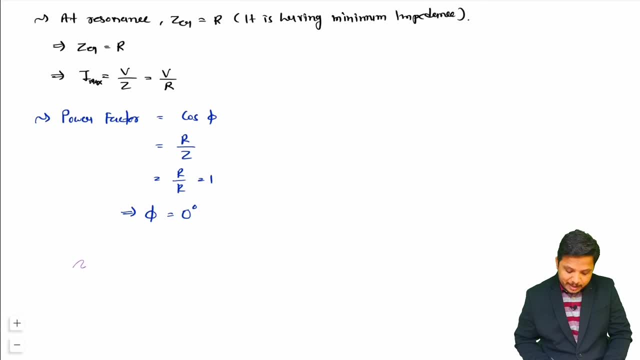 current that is 0, then you see what will happen here. if I say: this is my voltage phasor, and here I am drawing my current phasor, so both are overlapping over each other. and as both are overlapping over each other, you can say there will be maximum current which will flow. 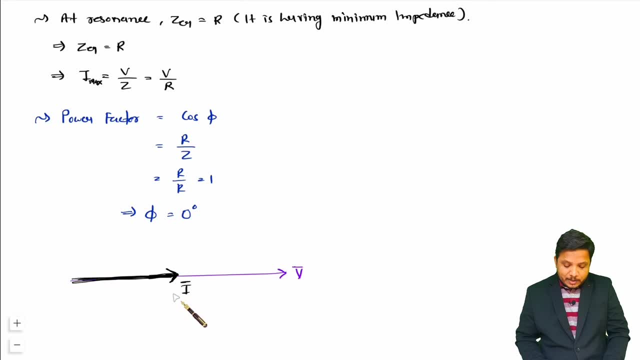 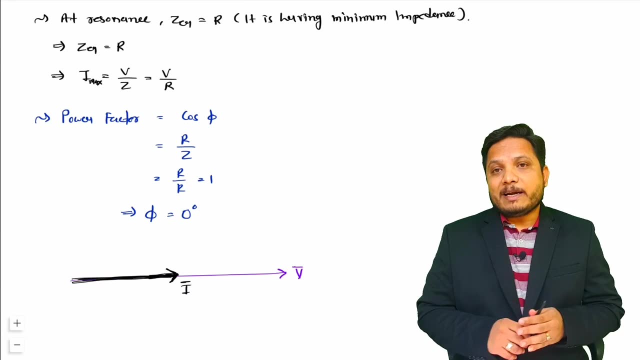 as well, as there will be resonance in which you will be having minimum impedance that is Z. equivalent is equals to R. So, my dear students, how many points that you should take care of here when you talk about resonance for series. This is a case of series Common. 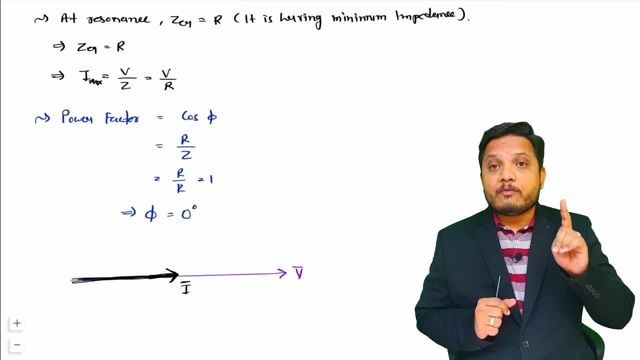 point is at resonance, phase of voltage and current will be same. So in case of series connection you will be having impedance calculation and for that you will be observing. imaginary component should be 0. in that case you will be having impedance calculation and for that case you can have voltage and current will be there in same phase At that time. frequency.